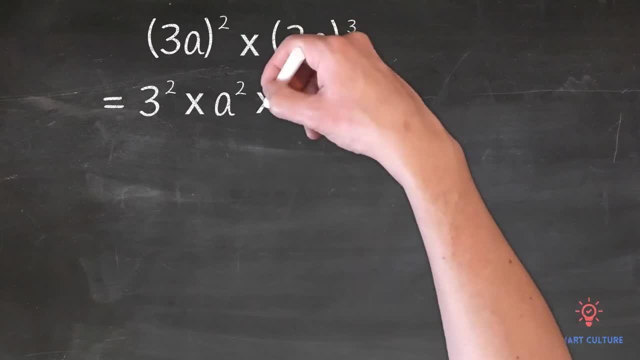 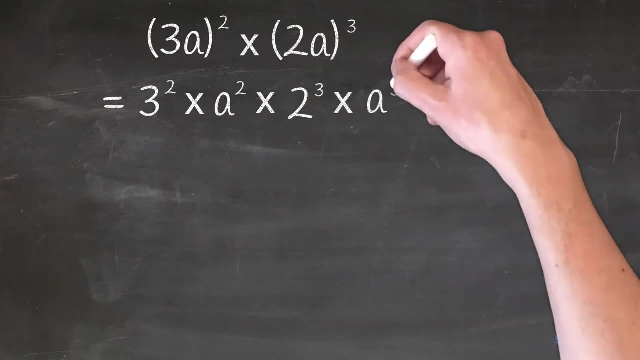 1, 1 times 2 equals 2.. This 2 has an exponent of 1, 1 times 3 equals 3.. This a has an exponent of 1, 1 times 3 equals 3.. So now we have 3 squared times a squared times 2 cubed times a cubed. 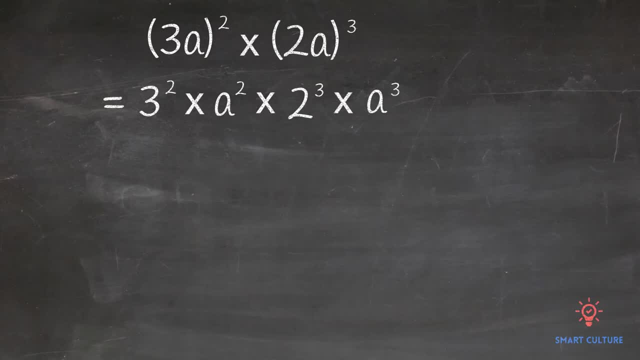 Remember, the product of powers of the same base is equal to the same base raised to the sum of the exponents of the powers. 3 squared is equal to 9.. a squared times a cubed is equal to a raised to the power of 2 plus 3.. 2 cubed is equal to 8.. Now we have to. 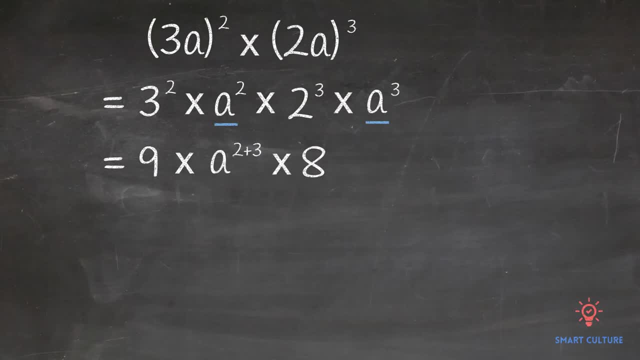 multiply 9 and 8.. That equals 72.. 2 plus 3 equals 5.. So the final answer will be equal to 72a, to the power of 5.. Take a look at the following example. So what we have to do now is we have to expand the brackets. 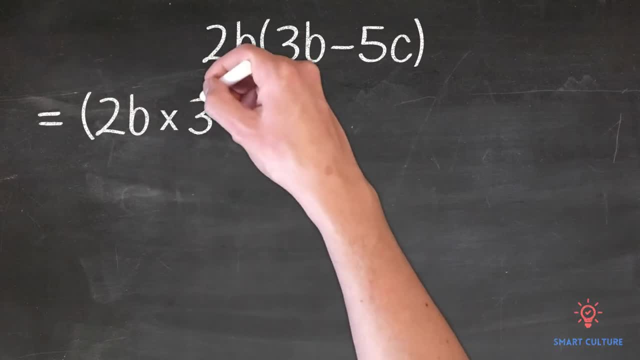 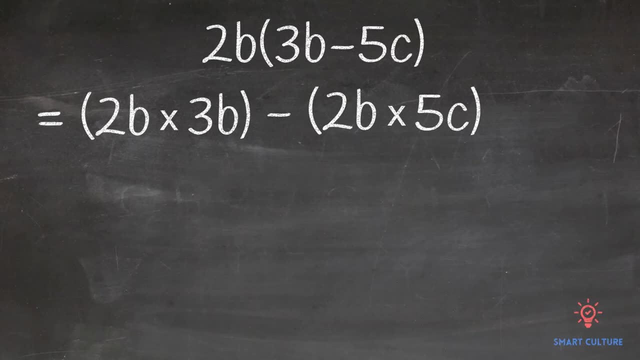 To expand a bracket means to multiply each term in the bracket by the expression outside the bracket. So let's start 2b times 3b minus 2b times 5c. So what we'll do now is we'll write it. 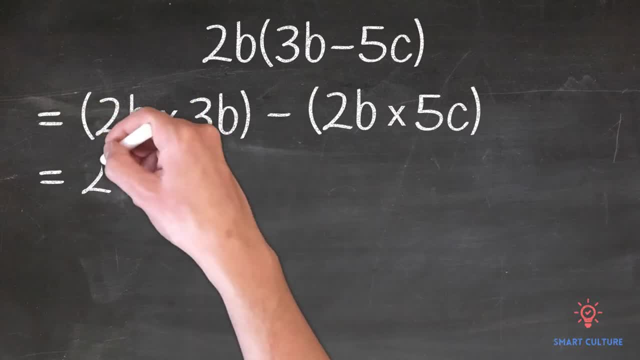 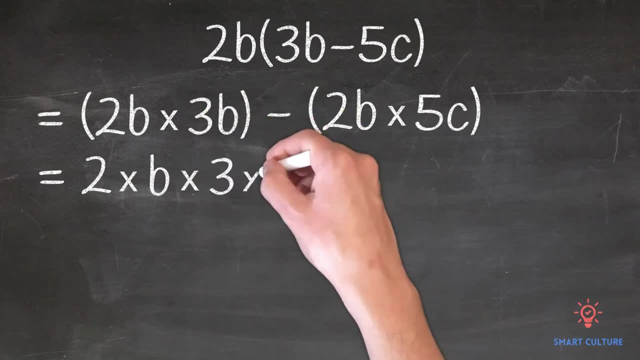 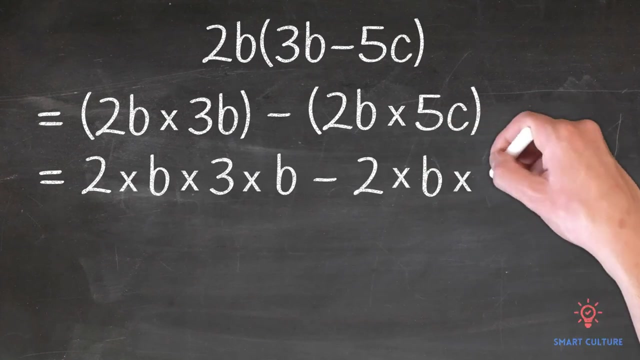 out in expanded notation. Let's start: 2 times b times 3 times b, minus 2 times b times 5 times c. Take a look at the coefficients. So first we'll multiply the numerical coefficients: 2 times 3 equals 6.. 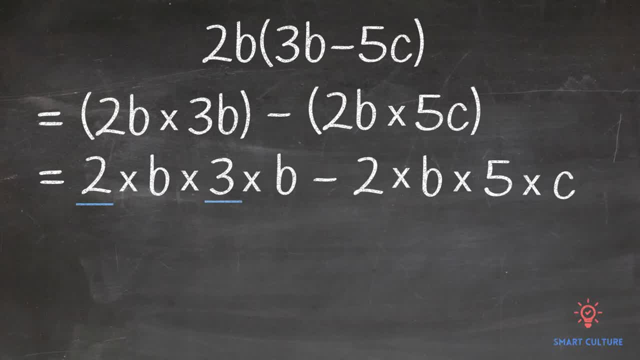 Then we'll multiply the variables: b times b is equal to b squared. Remember, the product of powers of the same base is equal to the same base raised to the sum of the exponents of the powers. Remember, a negative times a positive equals a negative. So negative 2 times 5 is equal to negative 10.. b times c is equal to bc.